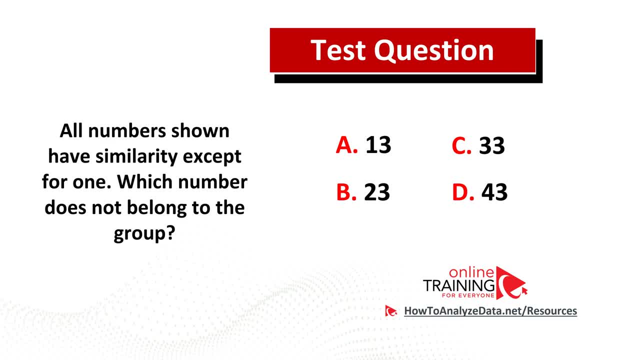 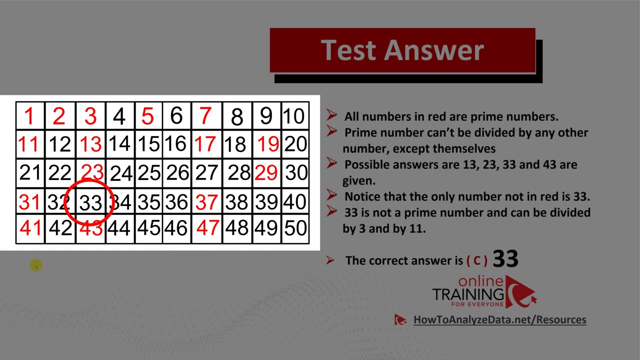 might be a good time to pause this video to see if you can come up with the answer on your own. Did you come up with the answer? Let's continue to see how we can solve this challenge together. The solution lies in understanding a very simple math concept, the concept of prime numbers. 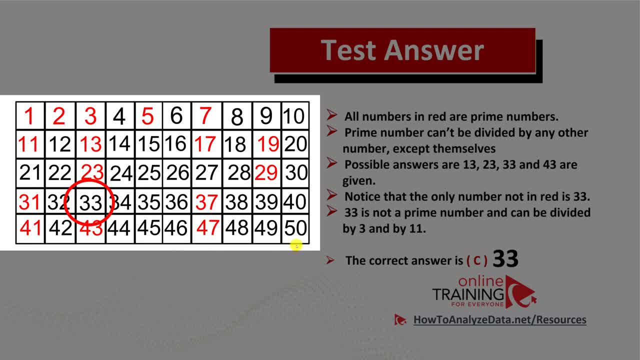 You see on the left the grid of numbers from 1 to 50.. And all the numbers that are considered prime numbers are highlighted in red. What is prime number? Prime number is the number that you can only divide by itself. You cannot divide it by any other number. For example: 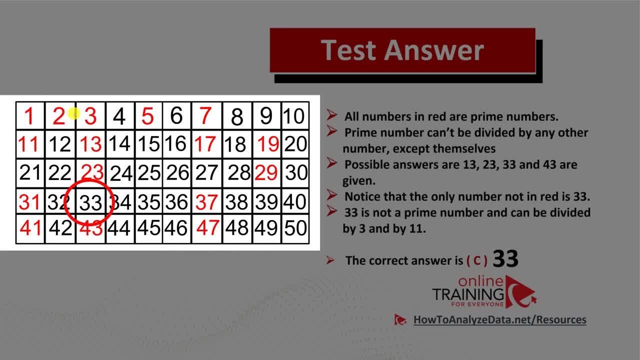 1. you cannot divide by anything but 1.. Same for 2,, 3,, 5,, 7, and etc. Out of all the numbers presented in the question, 33 is not a prime number, Because 33 can be divided by 3 and. 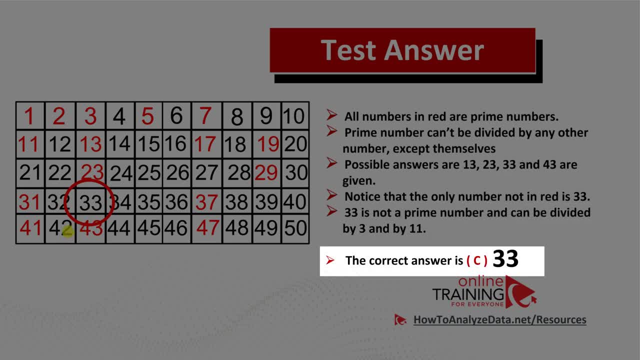 also can be divided by 11.. So the correct answer here is choice C 33.. Let's recap: All numbers in red presented in the grid are prime numbers. Prime number cannot be divided by any other number except themselves. Possible answers are 13,, 23,, 33, and 43. And the only number that is not a prime number. 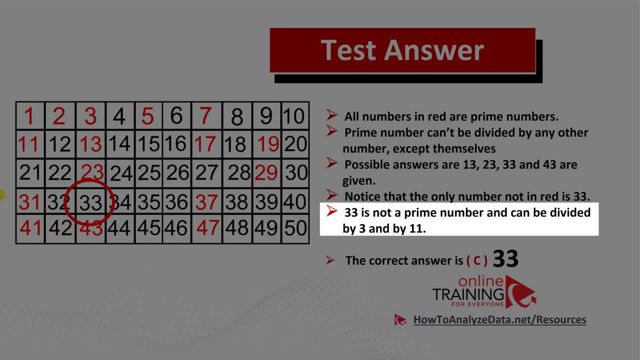 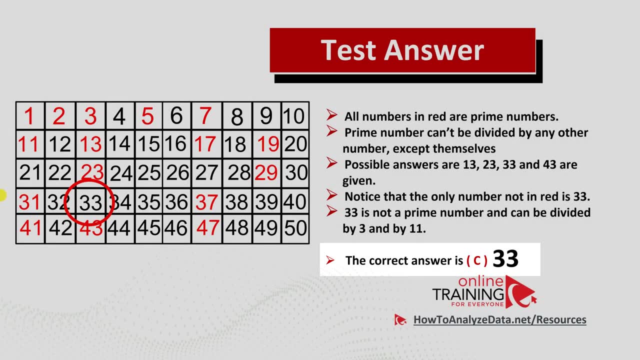 is 33.. 33 is not a prime number because it can be easily divided by 3 and by 11.. So the correct choice here is choice C 33.. Hopefully you've nailed this question and now know how to answer these types of questions on the test. 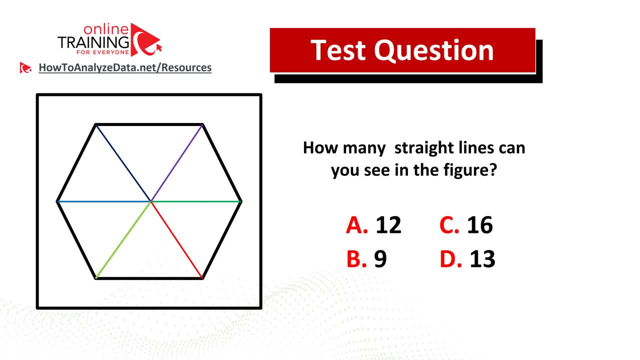 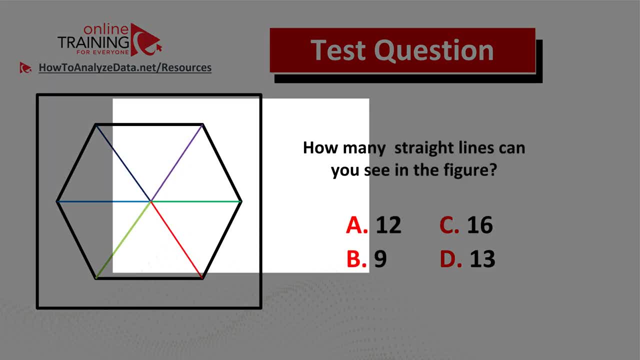 Here's the interesting and at the same time very tricky question you might frequently see on the test: How many straight lines can you see in this figure? In your presented was the figure on the left In your four different choices: choice A: 12 lines. choice B: 9,. choice C: 16, or choice D: 13 lines. Do you think you? 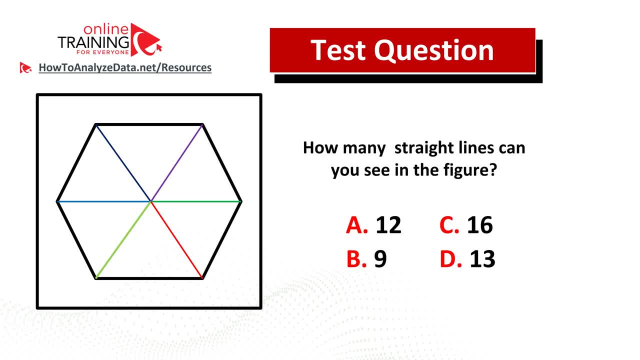 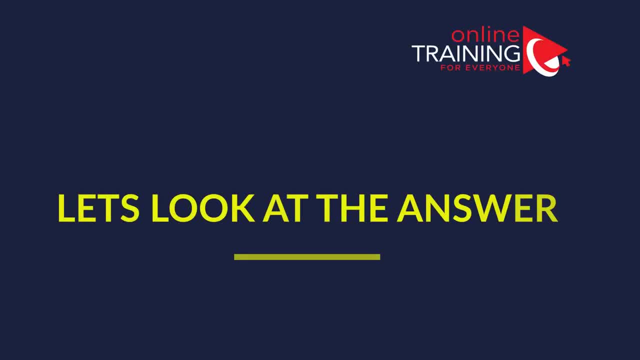 know the answer. Now might be a good time for you to pause this video and wait for possibly 20 to 30 seconds to see if you can come up with the answer on your own. Do you think you know the answer? Let's continue to see how we can solve this challenge and get to. 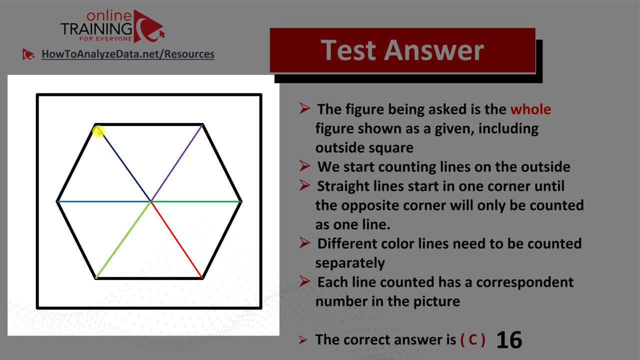 the solution together. The tricky part of this question is that we're not just looking at the inside shape and all the lines inside the inside shape, but also looking on the outside square shape. We start counting on the outside and I'm starting to count and by each line I'm putting. 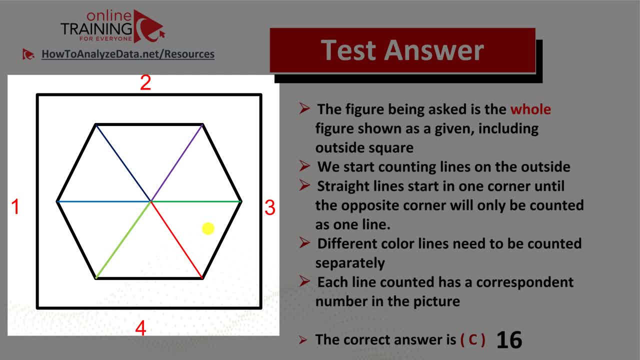 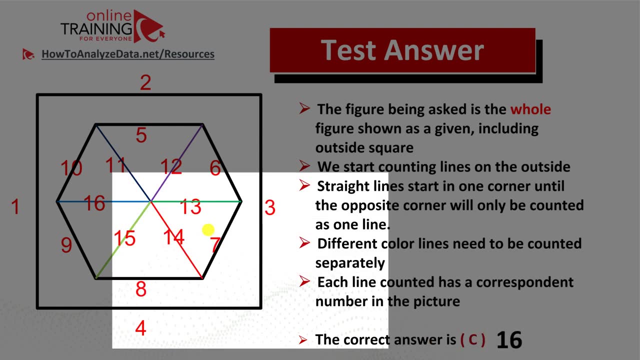 the number here. So outside shape has four different lines. Now let's count number of lines on the inside shape: 5,, 6,, 7,, 8,, 9,, 10,, 11,, 12,, 13,, 14,, 15, and then 16.. So the correct answer here is 16, 16 lines. 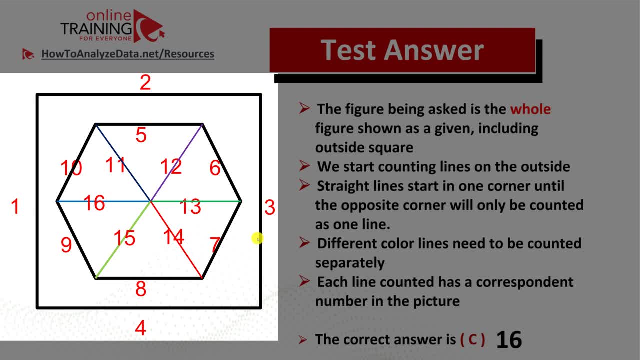 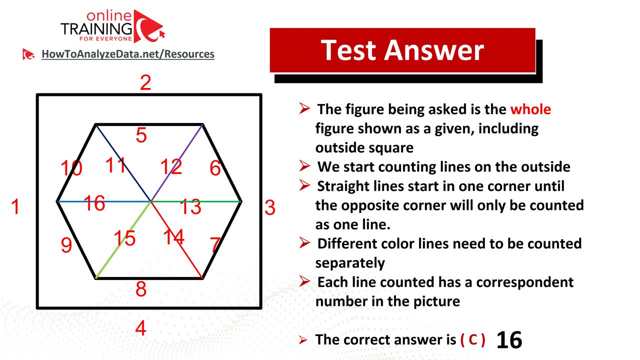 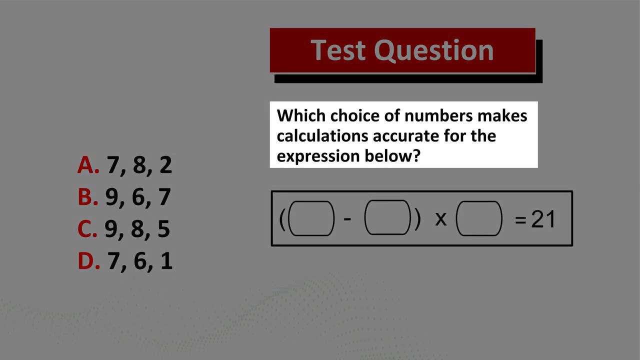 because that includes the outside shape, which has four lines as well. Hopefully you've nailed this question and now know how to answer similar questions on the test. And now here's the question for you to try: Which choice of numbers makes calculations accurate for the experiment? 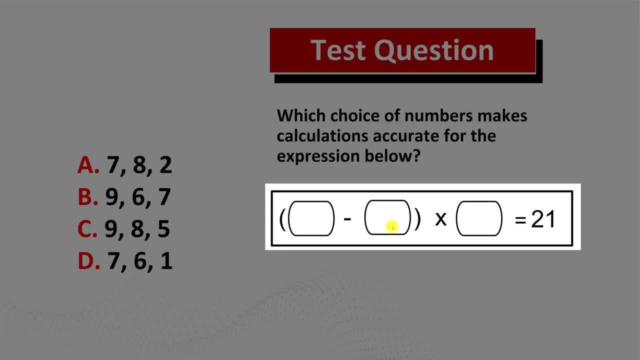 Here's the expression below And you have an expression: Two numbers in parenthesis multiplied by a third number equals 21.. And for two numbers in parenthesis you subtract second number from the first number And you have four different choices. Choice A: 7, 8, 2.. Choice B: 9, 6, 7.. 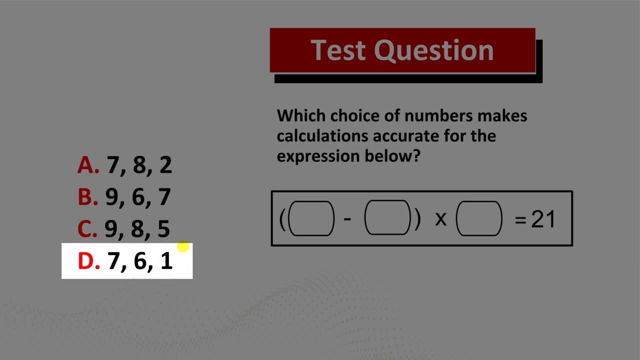 Choice C: 9,, 8, 5.. Or choice D- 7,, 6, 1.. Feel free to pause this video and try to solve it, And if you came up with the answer, feel free to pause. 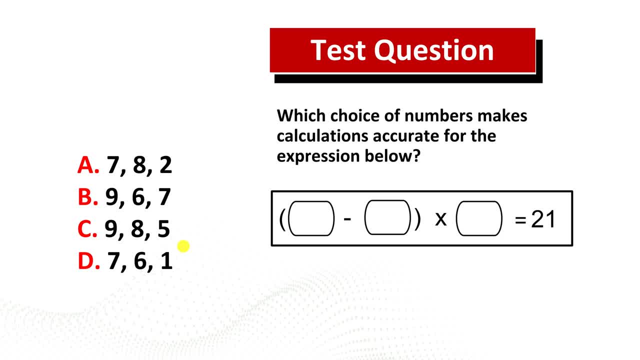 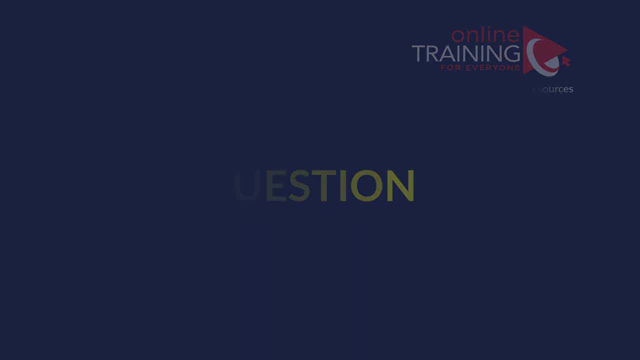 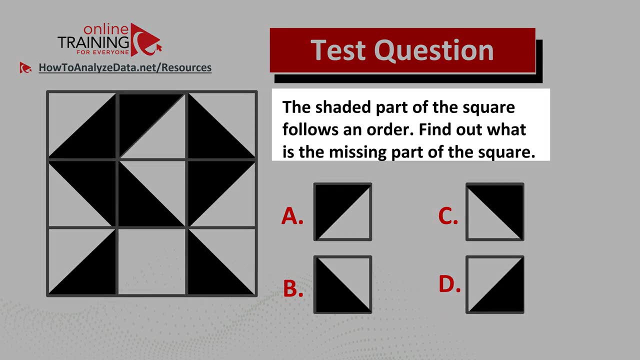 it in the comment section of this video and I'll give you my feedback. Thanks for participating. The question here is quite tricky, but I would like to show you the solution which, as you will see, is quite simple: The shaded part of the shape. follow the order. 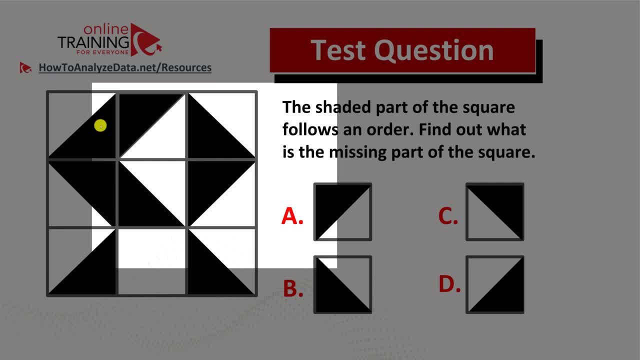 find out what is the missing part of the square And you're presented with the 3x3 square And one box inside the square, on the lower part in the middle, is missing. you need to pick a replacement square out of four possible choices: choice a, b, c and d. 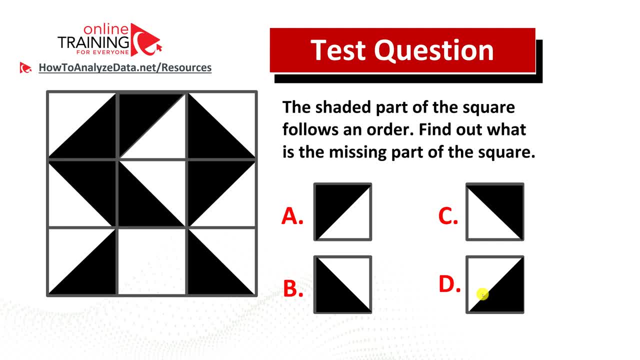 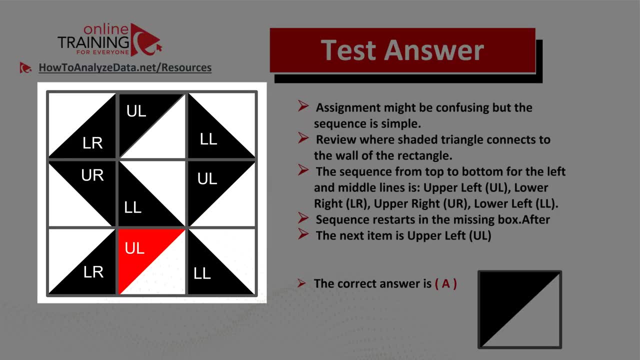 do you think you know the answer? now might be a good time to pause the video to see if you can come up with the solution on your own. do you think you know the answer? let's continue to see how we can solve this challenge together and get to the correct solution. as usual, to solve these types of questions, you need to look at the 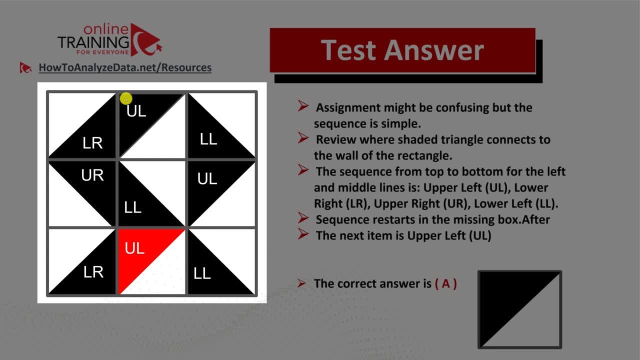 sequence. and sequence is determined by where inside dark triangle connects to the inside walls of the rectangle. so, for example, if you look at the left and middle line, this is where the sequence is. you see that it starts with upper left. so we have upper connection and then left. 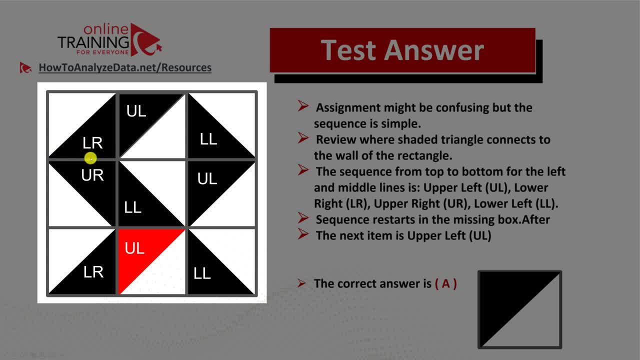 connection then goes to lower right, so we have lower connection and then right connection, then goes to upper right and then goes to lower left, and then this is the missing box where we need to find the missing square. and you see that the pattern here restarts. upper left was the first item in the sequence, so the next item in the sequence would be upper left. 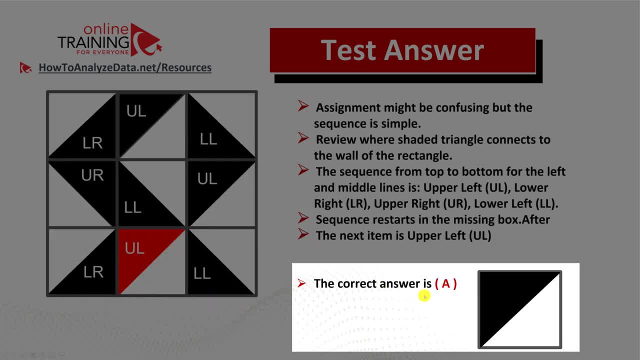 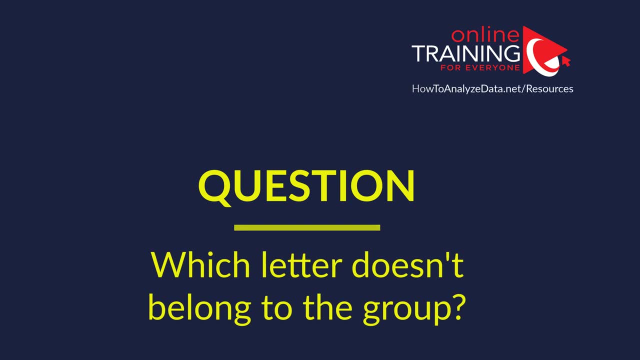 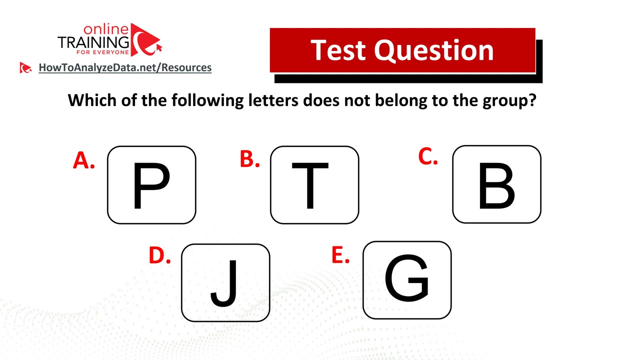 again. so the correct choice here is choice a upper left. hopefully you've nailed this question. some of you might find this question tricky, but regardless of whether you can solve it or not on your own, you will be excited to learn the solution to this real life assessment test question, which. 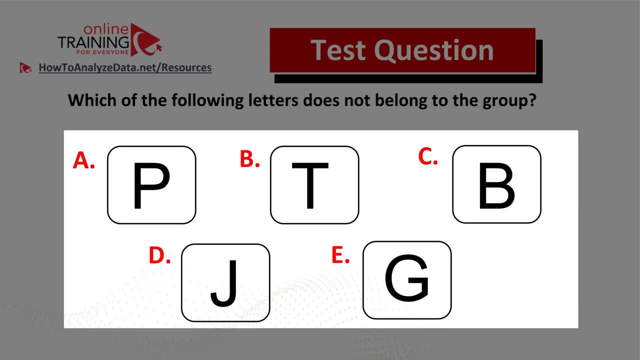 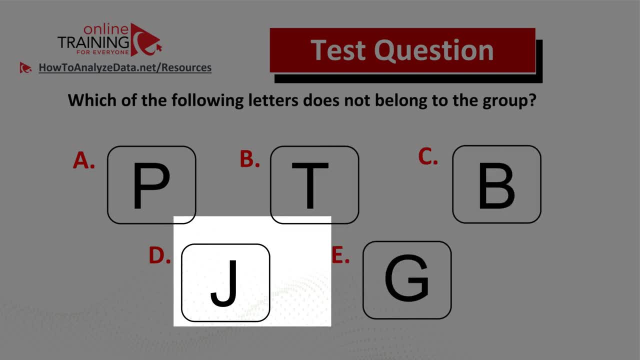 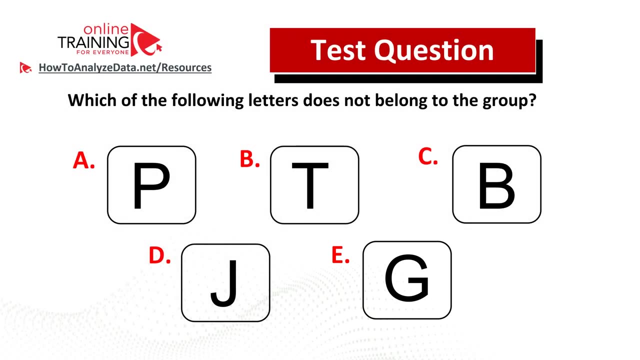 of the following letters does not belong to the group and you have five different choices: choice a- letter p, choice b- letter t, choice c- letter b, choice d- letter j and choice e- letter g. do you think you know the answer? now might be a good time to pause this video. 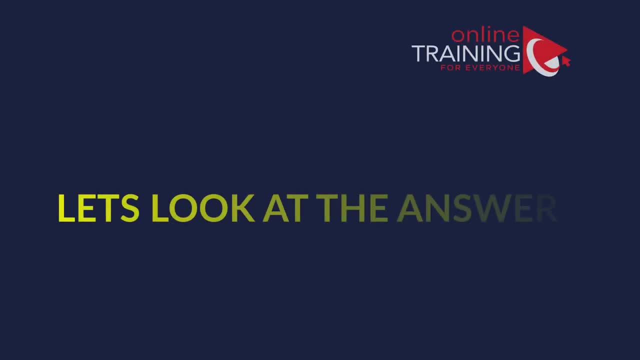 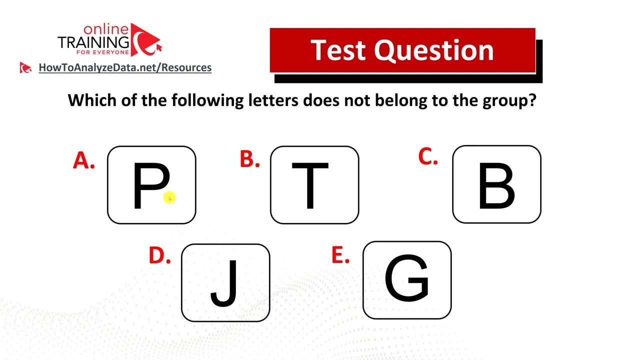 to see if you can come up with the answer on your own. let's continue you to see if we can solve this challenge and get to the solution together. before we jump to the solution, i would like to give you a clue: always look for patterns and the pattern here. 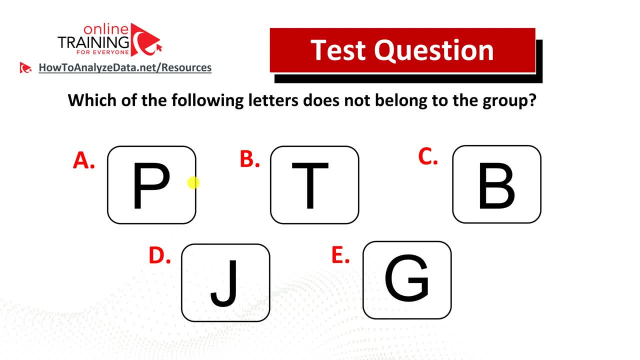 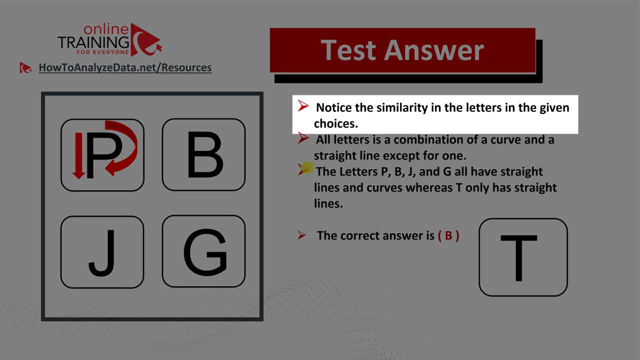 might be sharp edges versus rounded areas for the letters. now let's go ahead and jump to the solution. when you look at the patterns, you can notice the similarities in the letters for the given choices. all letters are combination of the curve as well as straight line, with the exception. 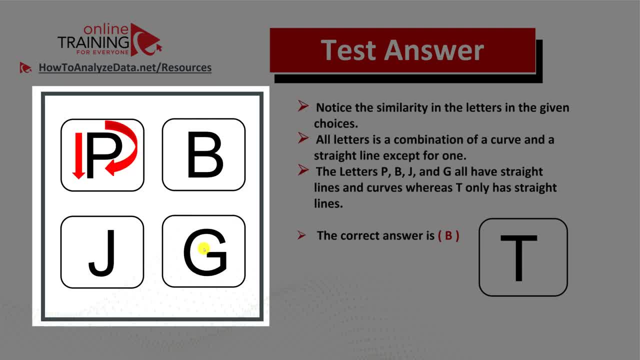 of one. the letters p, b, d and e are the same. these letters are the same, but as soon as we have the B, J and G presented here, they all have combination of curve as well as straight line. The only letter that does not match this pattern is letter T. 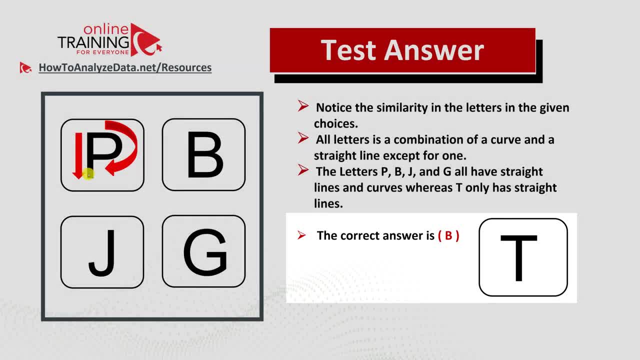 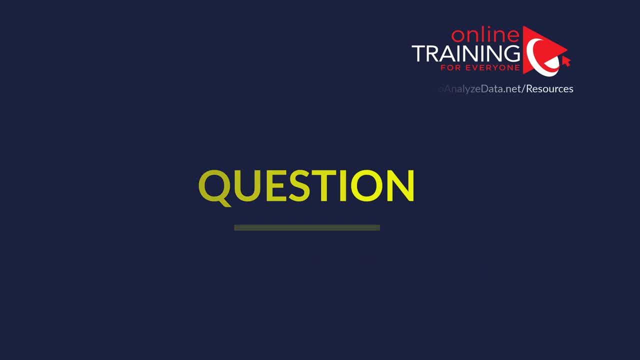 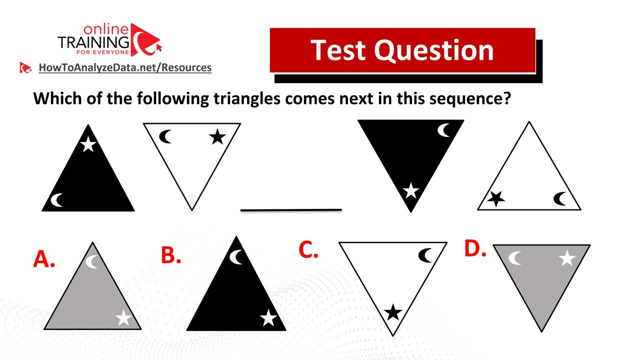 So the correct choice here is choice B, letter T. Hopefully you've nailed this question All right. I have a tricky question for you which you might frequently see on the test. The cool thing is that you might be able to solve it. 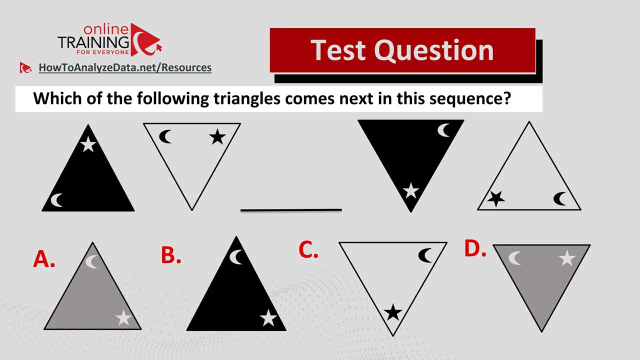 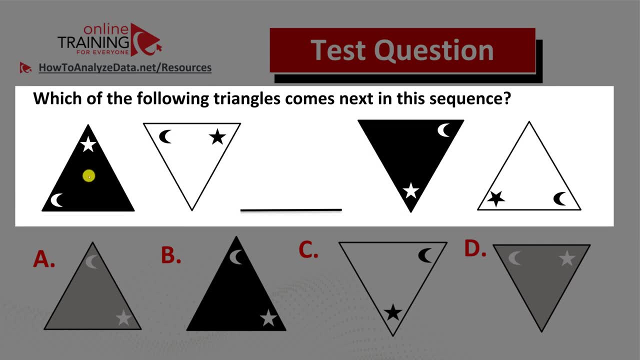 Or, in case you don't, I would love to show you the solution: Which of the following triangles comes next in the sequence? You have sequence of five triangles and one triangle in the middle is missing, And you have four different choices to pick the right triangle. 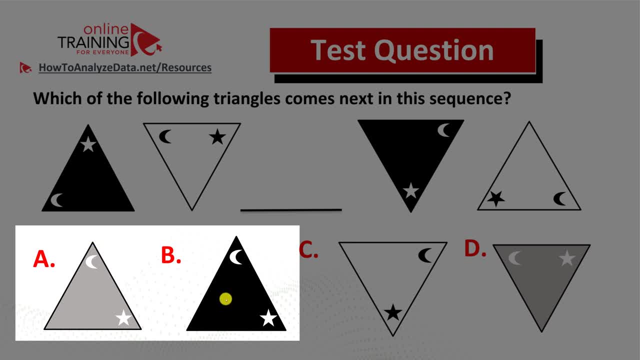 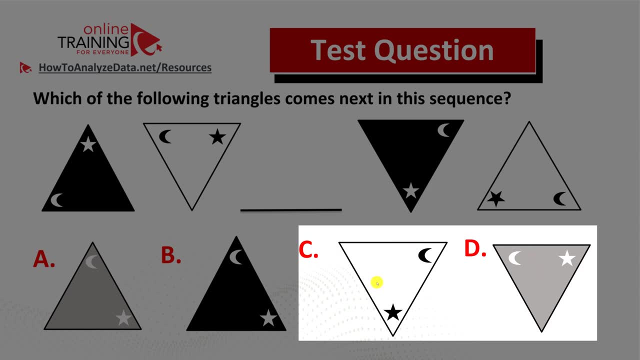 Choices A and B, represented by gray and black triangles pointing toward the top, And choices C and D, represented by white and gray triangles pointing to the bottom. Do you think you know the answer? Now might be the right time to point. Pause this video to see if you can come up with the answer on your own. 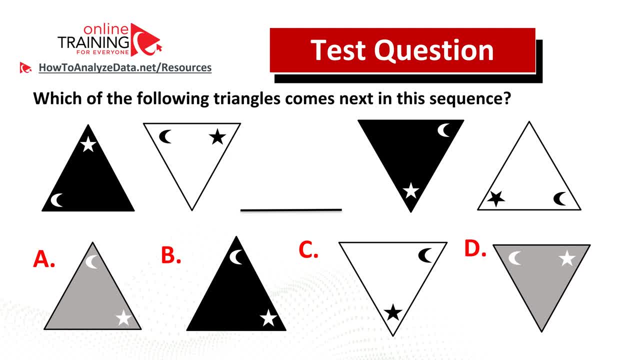 Do you think you came up with the answer? Let's continue to see how we can solve this challenge together. Before revealing the solution to you, I would like to point at two patterns that we see in this problem. The first is the pattern of colors. 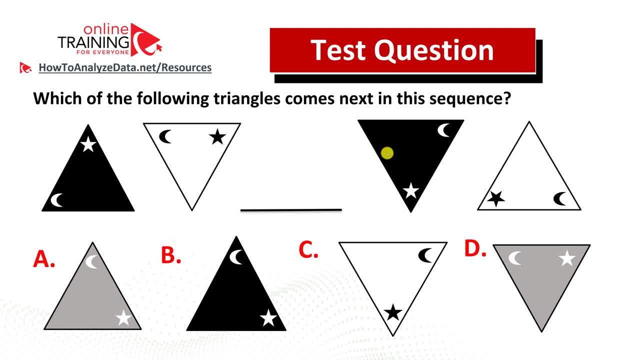 You have black triangle, white triangle and then missing triangle, then black triangle and white triangle, So something might be different from black and white. You also have a pattern of moon and star and moon and star. they move inside the triangle. 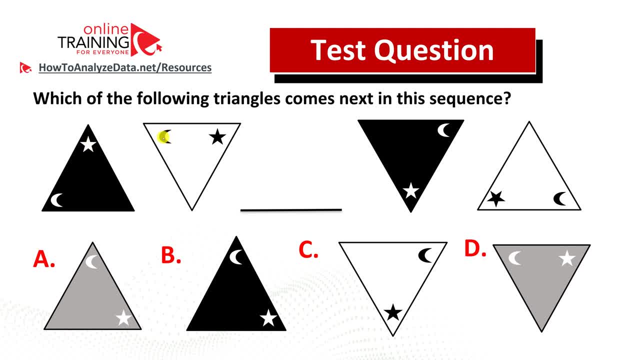 So you see moon and star in the leftmost triangle, then you see moon and star on the top, then you see moon on the top and star at the bottom, and then you see both of them: moon and star at the bottom of the triangle. 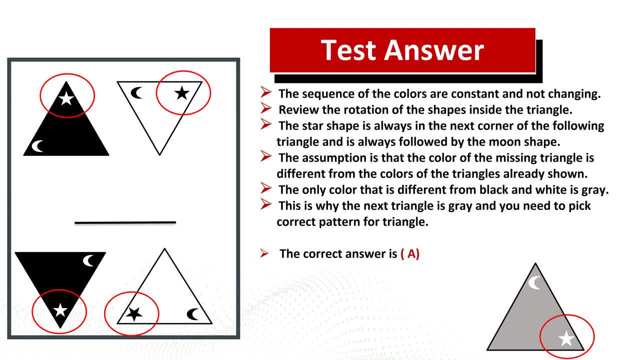 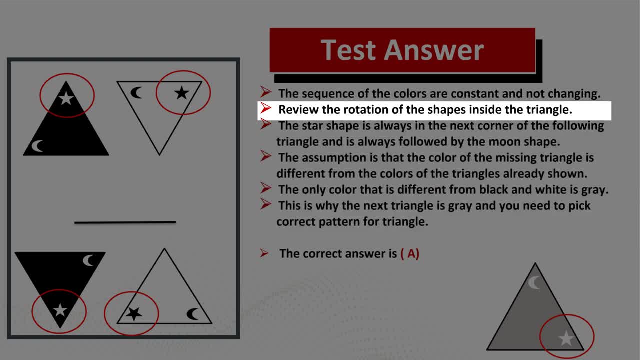 So now let's jump to the solution. We have already looked at the pattern of the colors, and the sequence of colors is constant And it's not changing. And we also reviewed the rotation of the shapes inside the triangle. The star shape is always in the next corner of the following triangle and is always followed by the moon shape. 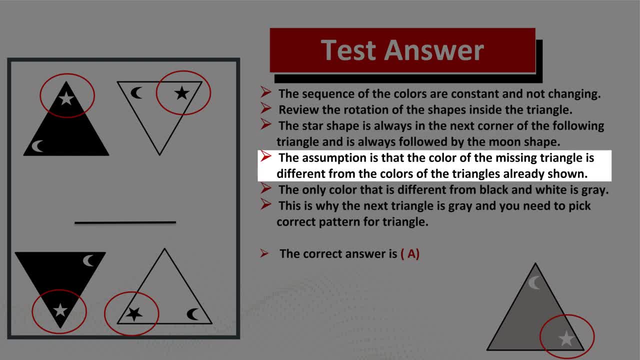 The assumption here is that the color of the missing triangle is different from the colors of triangles already shown, And the only color that is different from black and white is gray. This is why the next triangle is gray, and you would need to pick the correct pattern for the triangle. 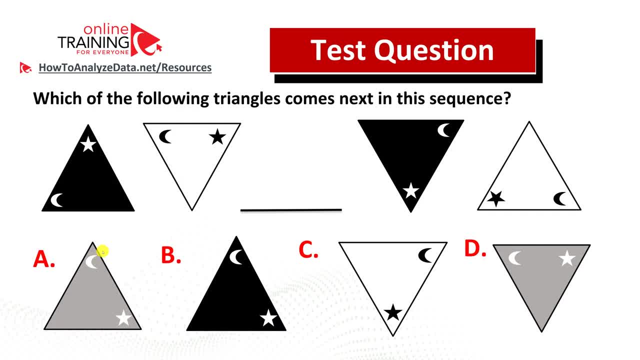 So the correct choice here is choice A. There are two gray triangles here, choice A and choice D, But there is also a third pattern pattern that I did not mention because it will make things very obvious, And this is the pattern of pointing. 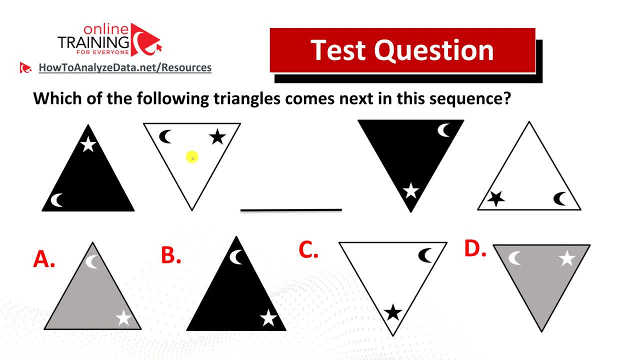 You see that the first triangle is pointing upward, The second triangle points down, So the next triangle in the pattern will be pointing up as well, And the only gray triangle that points up is choice A. Hopefully you've nailed this question and now know how to see the patterns. 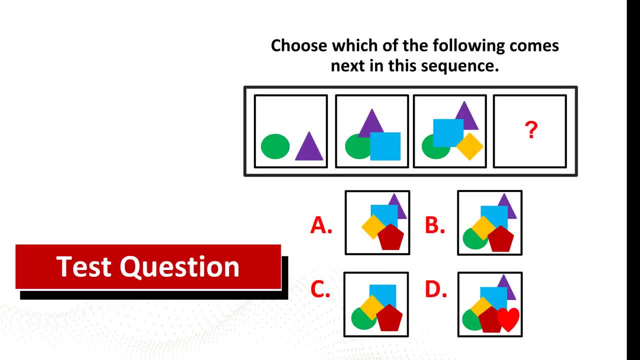 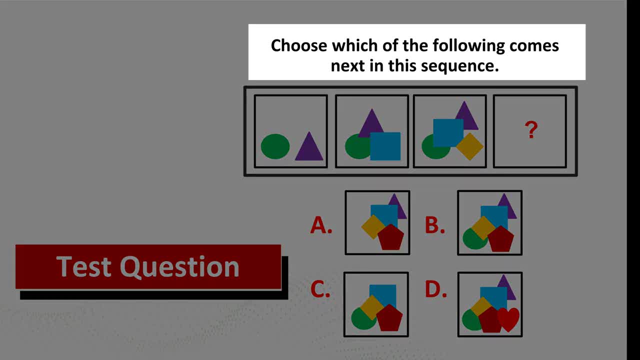 and solve this type of problem. And now here's the question for you to try. Please choose which of the following comes next in the sequence: You are presented with the sequence of objects And the fourth object in the sequence is missing, And you have four different choices presented here. 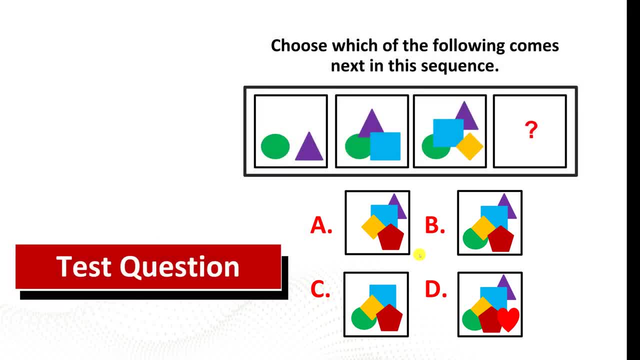 and you need to select one out of four choices. Feel free to pause this video and try to solve this challenge. Did you come up with the answer? Feel free to post it in the comment section below And if you have any questions, please leave a comment in the comment section of this video. 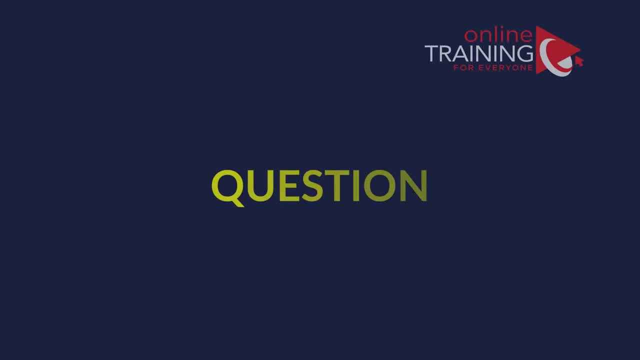 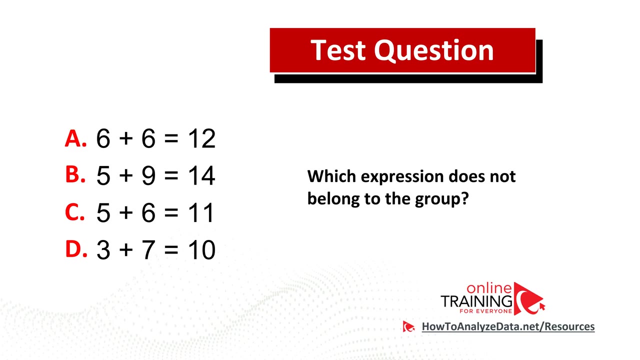 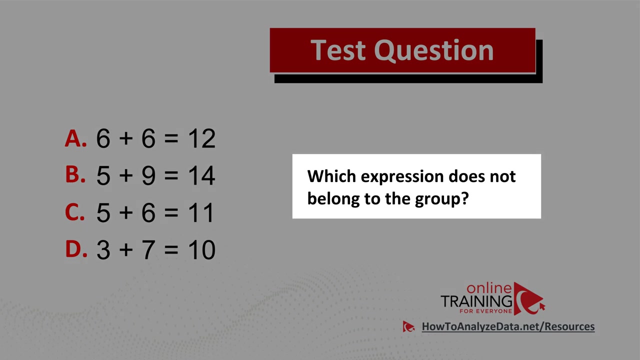 and I'll give you my feedback. Thanks for participating. Let's see if we can solve this challenge together. Here's the very interesting and at the same time tricky question you might frequently see on the test: Which expression does not belong to the group. 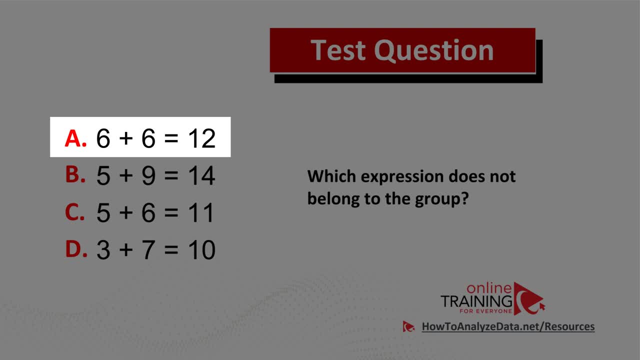 And you have four different choices: Choice A: 6 plus 6- equals 12.. Choice B: 5 plus 9- equals 14.. Choice C: 5 plus 9 equals 14.. Choice D: 5 plus 6- equals 11.. 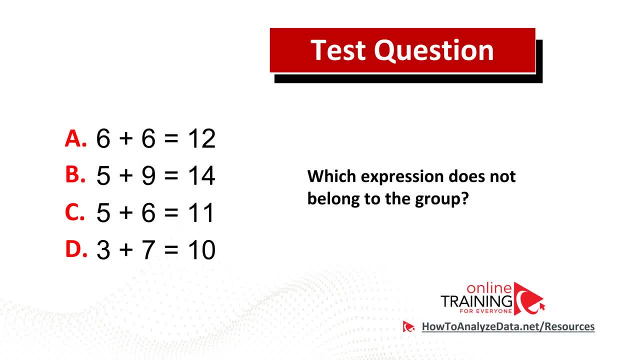 And choice D, 3 plus 7 equals 10.. Do you think you know the answer? Now might be the right time to pause this video to see if you can come up with the answer on your own. Give yourself 10 or 20 seconds. 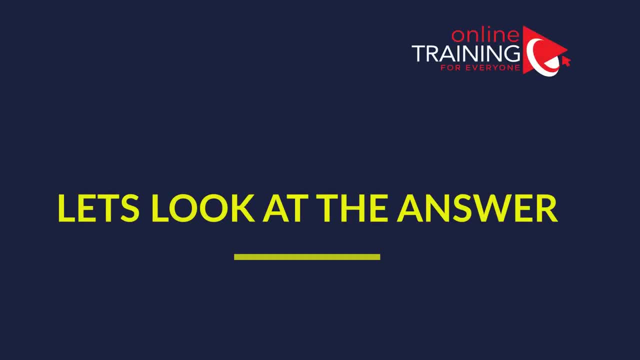 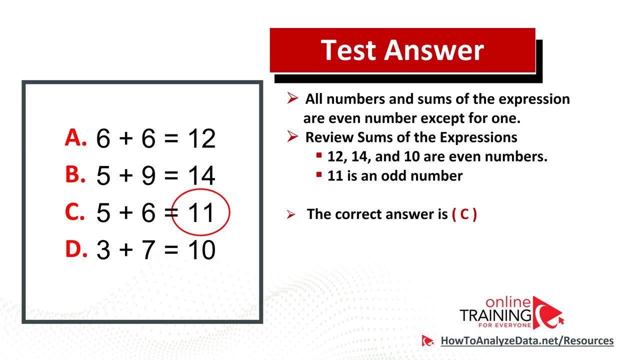 and see if you can come up with the solution. Did you come up with the answer? Let's continue to see if we can solve this challenge together. Let me show you two ways you can solve this challenge. First, let's look on the right side of the expression. 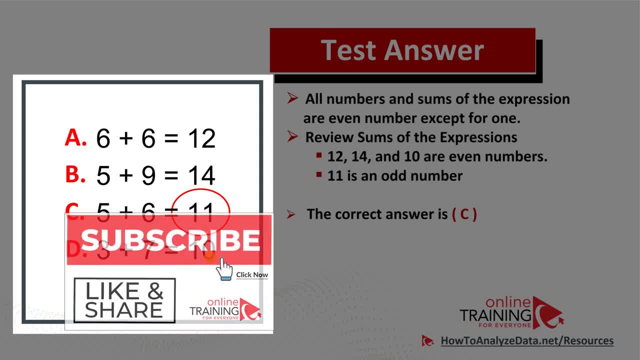 You see that the 12, 14 and 10 are all even numbers and 11 is the odd number. So that should give you some clues. If you look on the left side of the expression, you see that 6 plus 6 is the combination of even numbers. 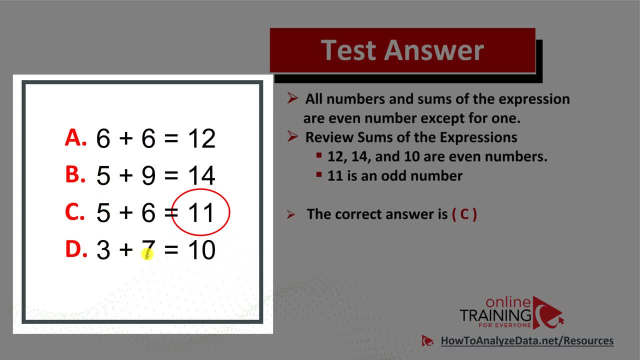 And you see that 5 plus 9 and 3 plus 7 is the combination of odd numbers. So expression C stands out because you have a combination of odd and even numbers in the choice C. So the correct answer, as you might have figured out, is choice C. 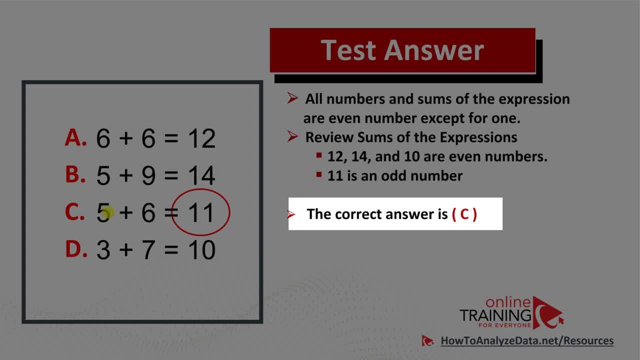 And there are multiple ways how you can look for clues to solve these types of challenges. Let's recap: All numbers in the sums of the expression are even numbers except one. If you review the sums of the expressions, you see that 12,, 14 and 10 are all even numbers and 11 stands out. 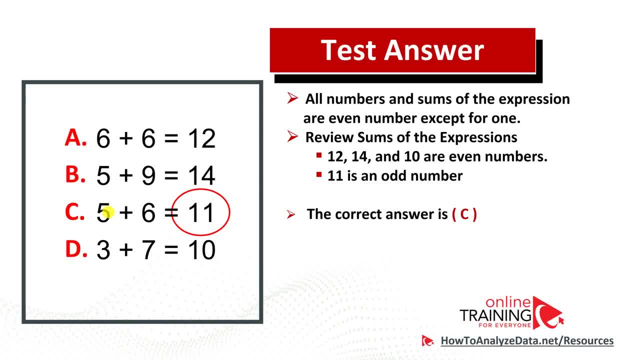 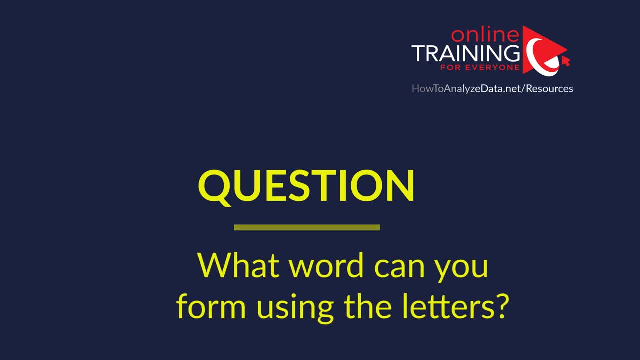 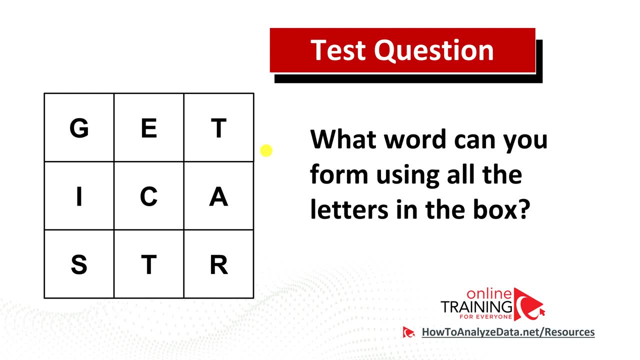 It's an odd number, So the correct answer here is choice C. Hopefully you've nailed this question. Let's look at the very interesting and at the same time, tricky question you might frequently see on the test. This particular question tests your imagination. 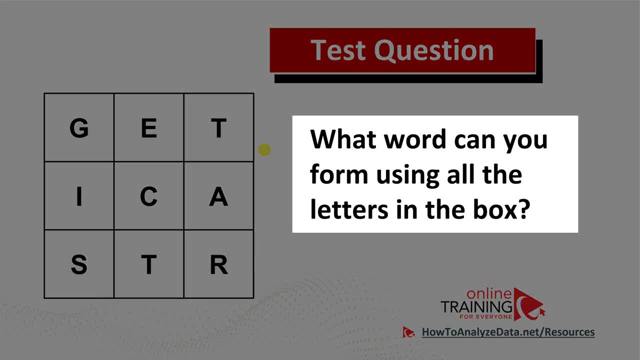 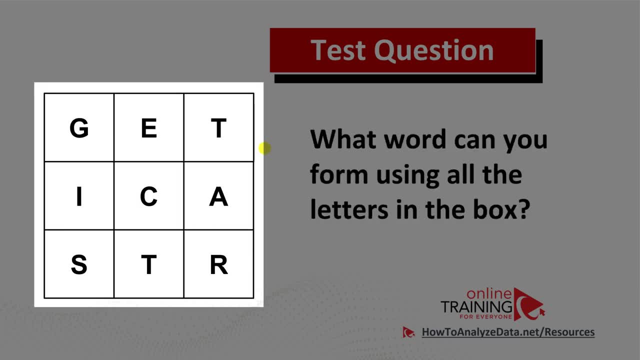 as well as the knowledge of the English words. What word can you form using all the letters in the box And you have nine unique letters presented in nine different boxes? Do you think you know the answer? Before we jump to the solution, this might be the right time for you to pause this video. 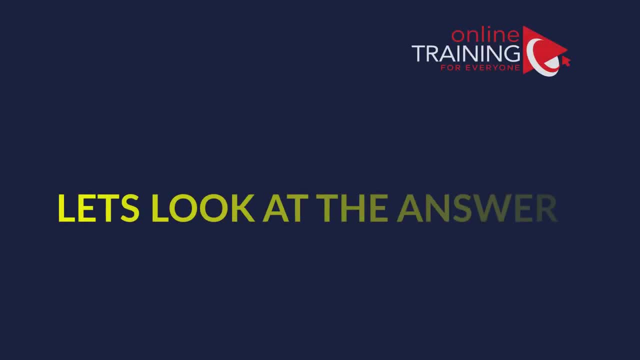 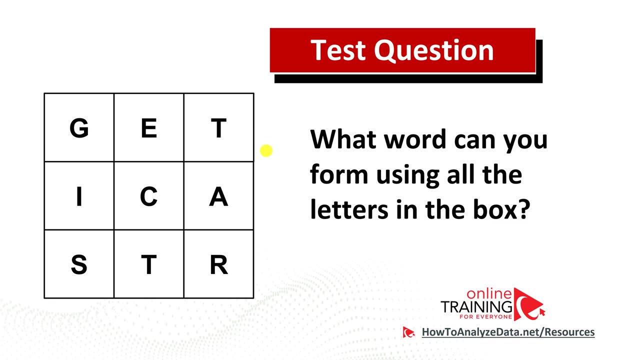 to see if you can come up with the solution on your own. Do you think you figured out the answer? Let's continue to see if we can solve this challenge together. Obviously, there are a lot of different words that could be formed with the given letters. 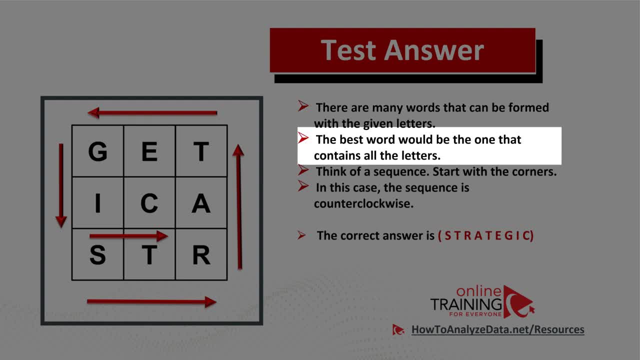 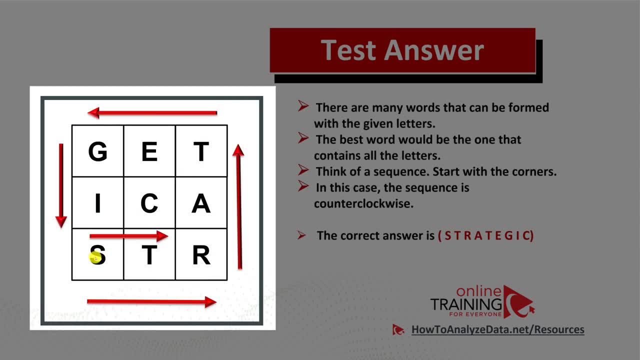 But what you need to do as part of the test is to find the word that best matches all the letters presented. You should start looking in the corners, And in this case the pattern is counterclockwise. We have the word strategic. 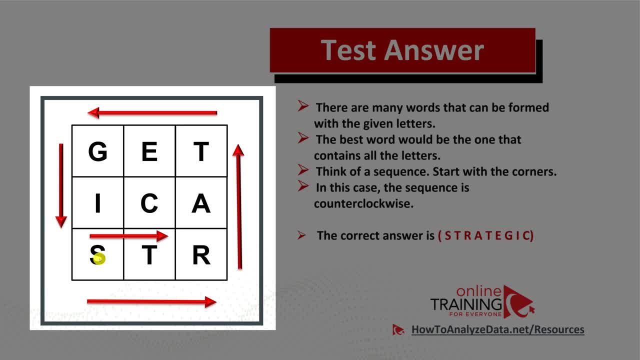 which is formed starting in the bottom left corner. If you start in the bottom left corner and then flow from right to left, then flow from bottom to the top, from left to right and then end your word in the middle, you will form the word strategic. 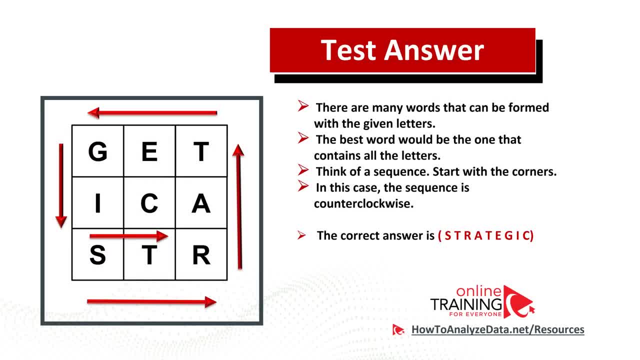 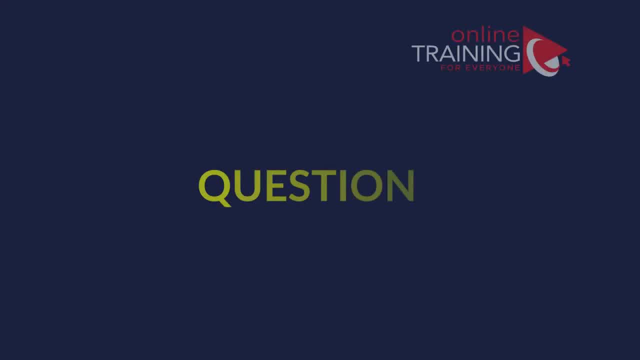 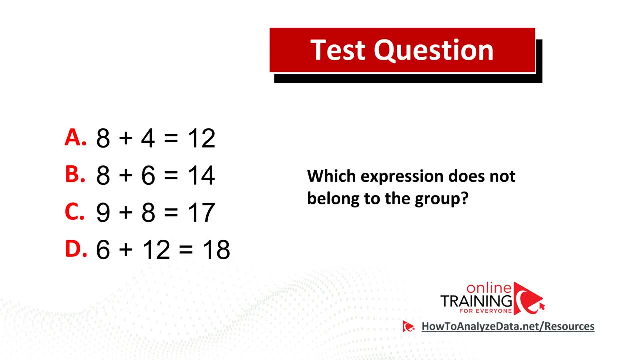 Hopefully you've nailed this question, But in case you need more questions or practice problems, please make sure to check out the aptitude test book in the description section of this video. Are you ready for this challenging problem? Let's look at the very first one. 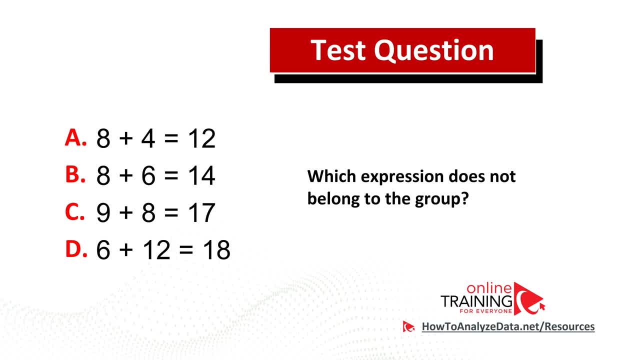 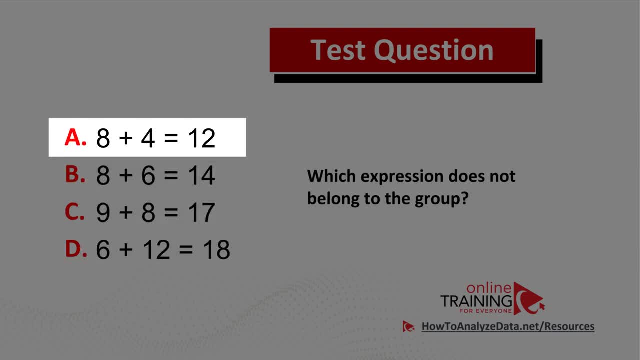 It's a very interesting and tricky question. you might frequently see on the test Which expression does not belong to the group And you have four different expressions. Choice A: 8 plus 4 equals 12.. Choice B: 8 plus 6 equals 14.. 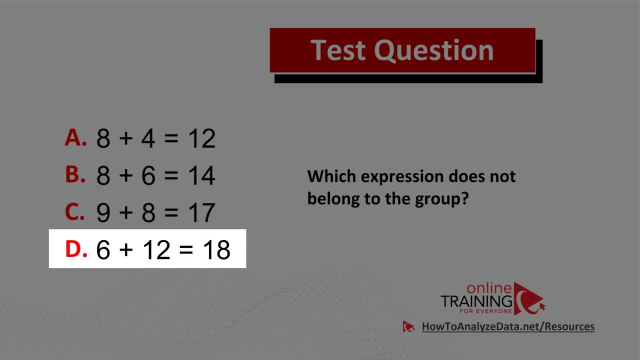 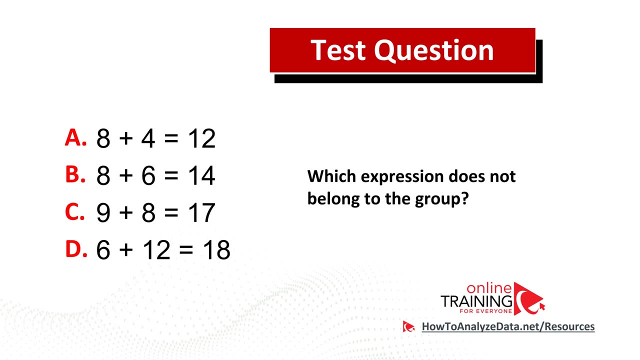 Choice C: 9 plus 8 equals 17.. And choice D- 6 plus 12 equals 18.. Do you think you know the answer? Now might be the right time for you to pause the video to see if you can come up with the answer on your own. 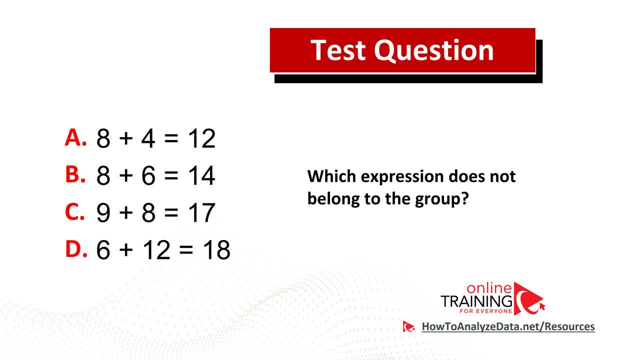 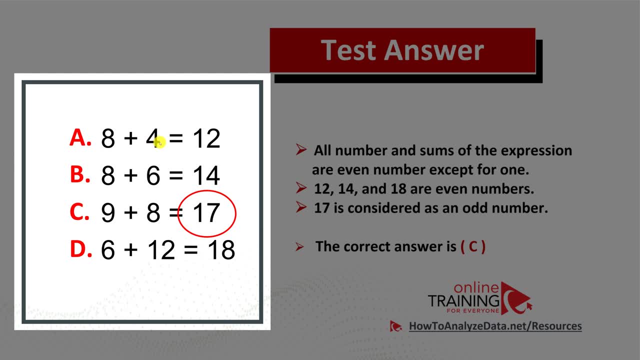 Do you think you know the answer? Let's continue to see if we can solve this challenge together. What's interesting about this question is the fact that we're dealing here with odd versus even numbers. You see that expression A has all the even numbers. 8 and 4 equals 12.. 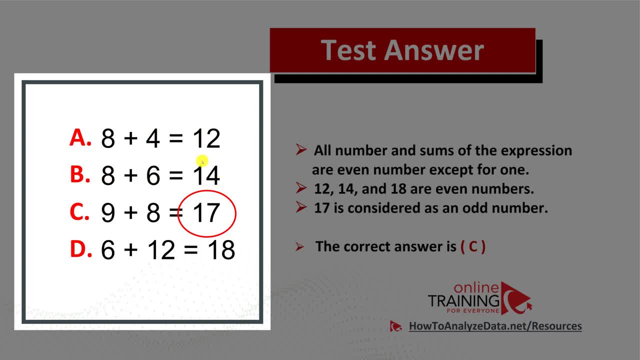 Expression B is the same thing. 8 plus 6 is 14, all even numbers Same with expression D: 6 plus 12 equals 18.. So the expression C has two odd numbers, 9 and 17.. If you look at the answers, you can also figure it out by just looking at the answer. 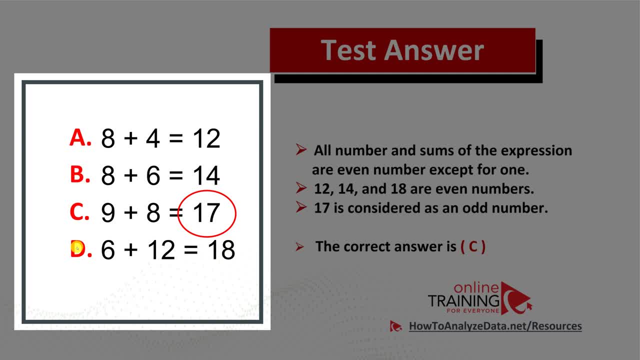 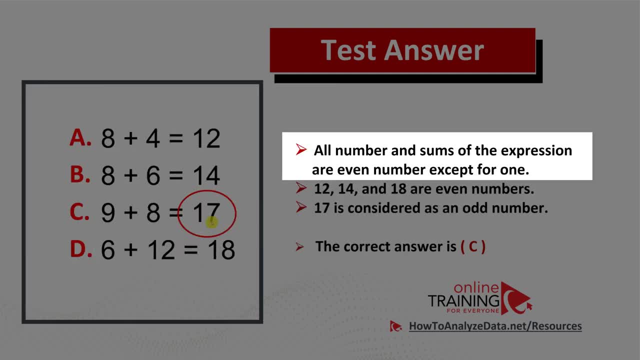 The answers are 12,, 14, and 18 for solutions A, B and D And for the C the answer is 17.. So let's recap. All numbers and sums of the expression are even numbers with the exception of one. 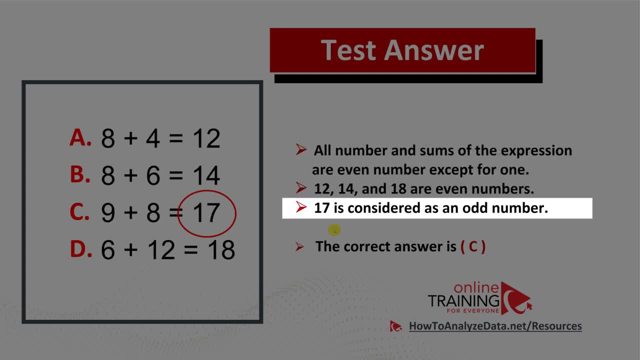 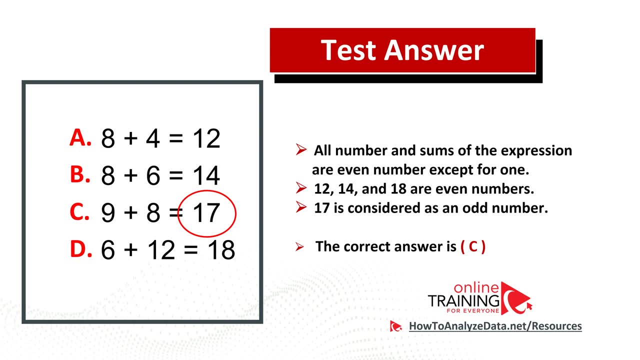 12,, 14, and 18 are even numbers, but 17 is the odd number, So the correct answer here is choice C 17.. Hopefully you've nailed this question and got to the correct answer on your own, But in case you need more questions or practice problems, 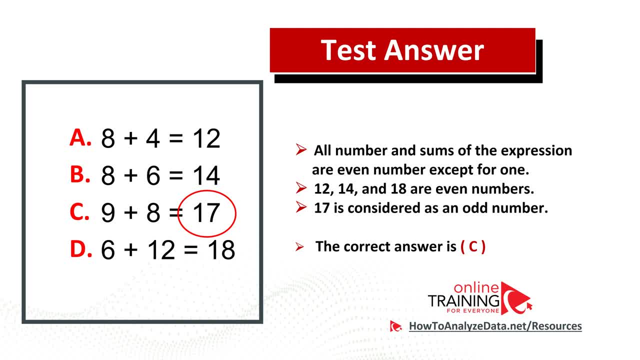 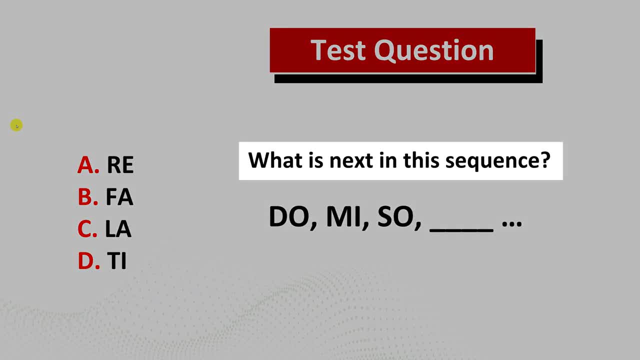 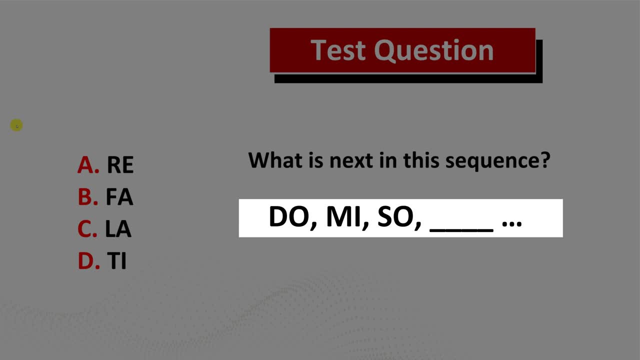 please make sure to check out the description of this video for my aptitude test questions PDF ebook. And now here's the question for you to try: What is the next item in the sequence- And you have series of items, Do me so. and then the next item that you need to determine. 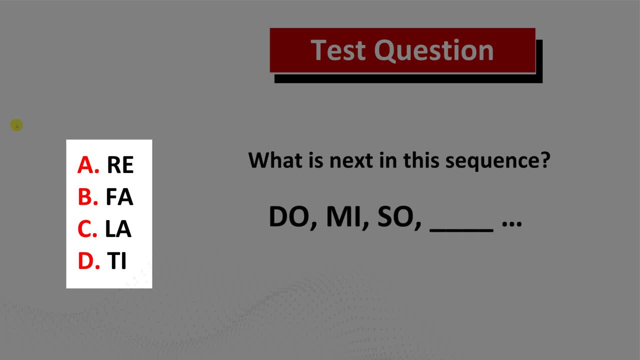 And you have four choices: Re fa la ti. Do you think you know the answer? Feel free to put your answer in the comments, Feel free to pause this video and try to solve it. And if you came up with the answer, 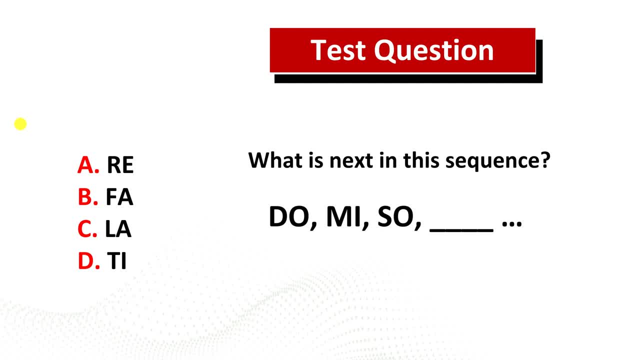 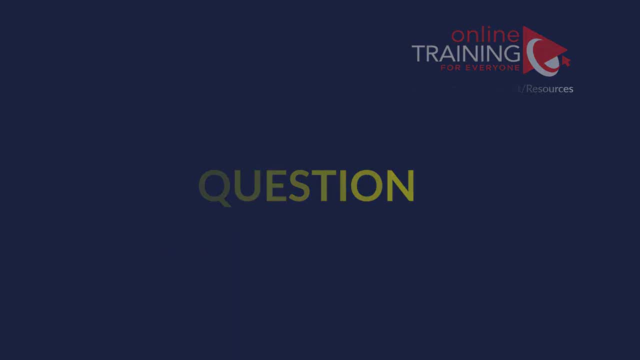 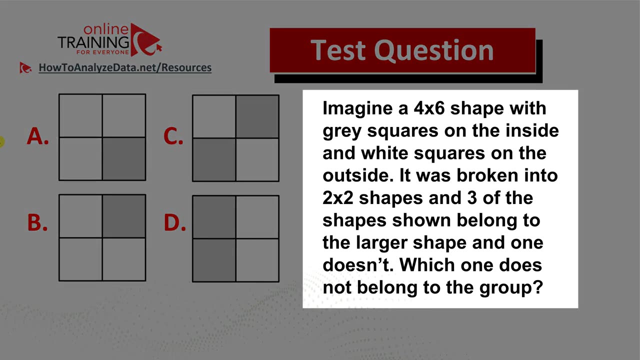 feel free to post it in the comment section of this video and I'll give you my feedback. Thanks for participating. Here's the tricky IQ and aptitude test question you might frequently see on the test. Imagine a 4x6 shape with gray squares on the inside and white squares on the outside. 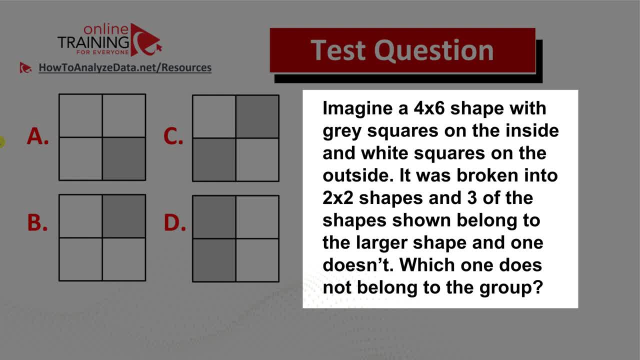 It was broken into 2x2 shapes and three of the shapes were broken. The shapes shown belong to the larger shape and one doesn't. Which one does not belong to the group? Do you think you know the answer? Now might be the right time to pause this video to see if you can come up with the answer on your own. 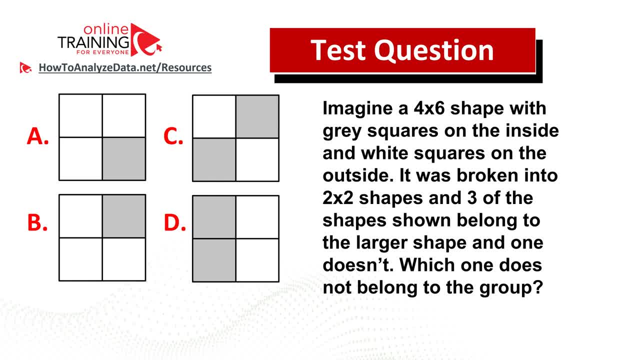 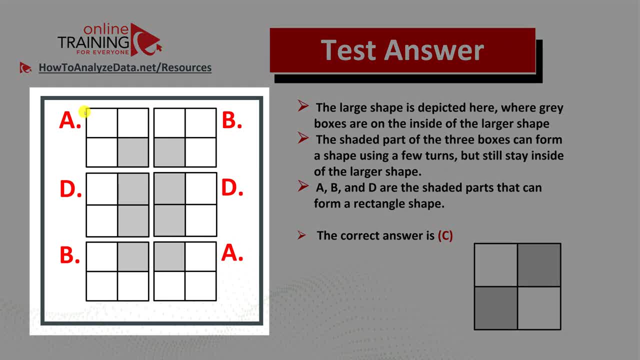 Do you think you came up with the answer? Let's continue to see if we can solve this challenge together. As you might be well aware, a visual is worth 1000 words or more. In this case, this is the shape. 4x6 shape. 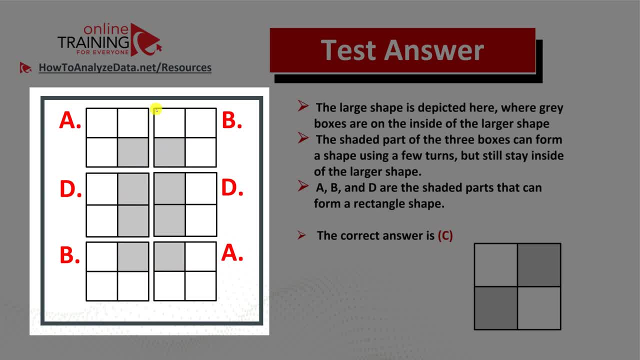 with the gray boxes on the inside and the white boxes on the outside, And it was broken down into 2x2 shapes. If we go back to the question, you see that the choice A is represented right here If you flip the box in the bottom right corner of the screen. 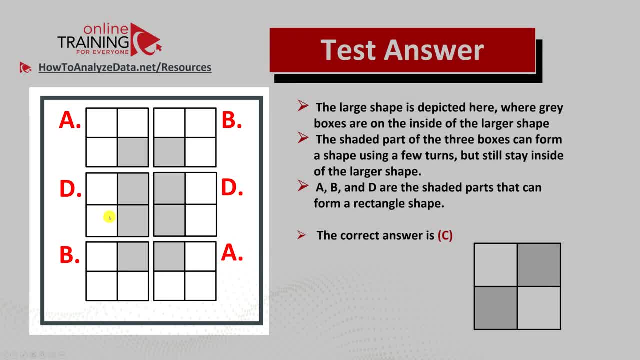 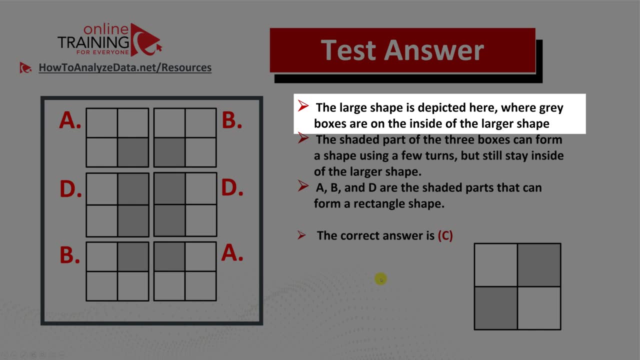 choices B are in the opposite corners and choices D are in the middle, But what you see is that choice C is not represented here anywhere, So the correct answer here is choice C. Let's recap: The large shape is depicted right here, where gray boxes are on the inside and the white boxes are on the outside of the larger shape. 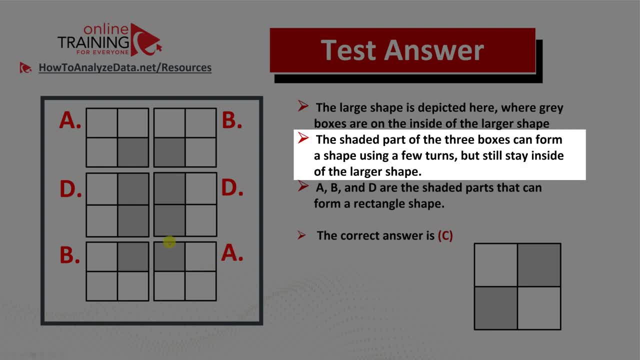 The shaded part of three boxes can form a shape using few turns, but still stay inside the larger shape. This is why choices A, B and D are valid choices and choice C is the correct choice, and this is the one you should be selecting. 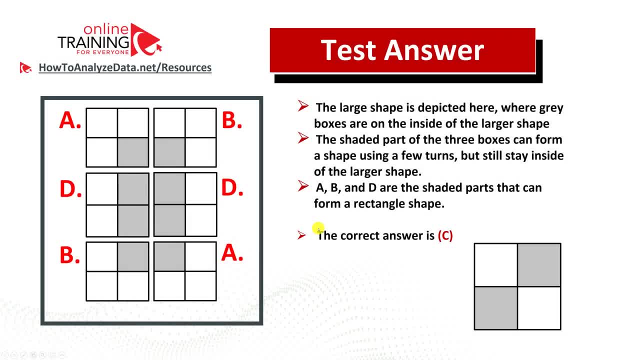 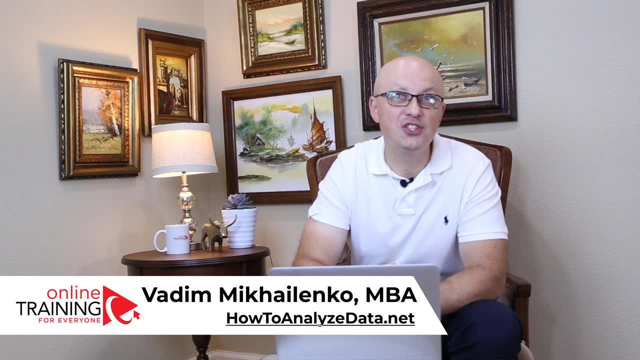 Hopefully you've nailed this question and answered it correctly, But in case you need more questions or practice, please make sure to check out my aptitude test question books in the description of this video. Thanks for watching. I encourage you to check out our daily question challenge in the community section of this channel. 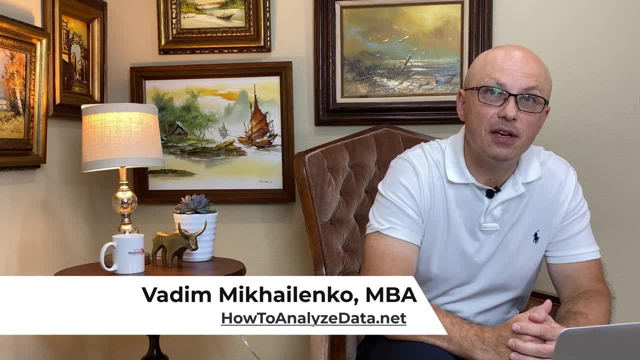 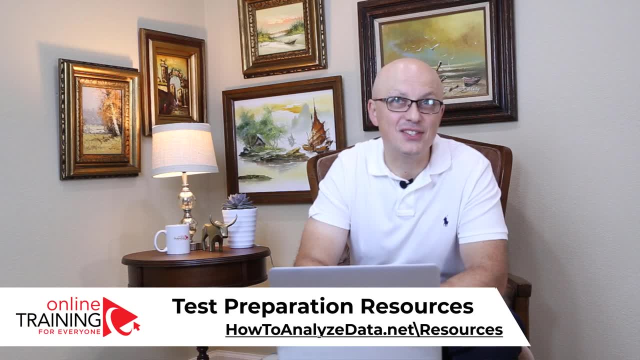 I also recommend that you check downloads in the description section of this video. Please also check out resources page on our website, howtoanalyzedatanet resources. If you like the content, please give this video a big thumbs up. This tells us that you need more content like this.